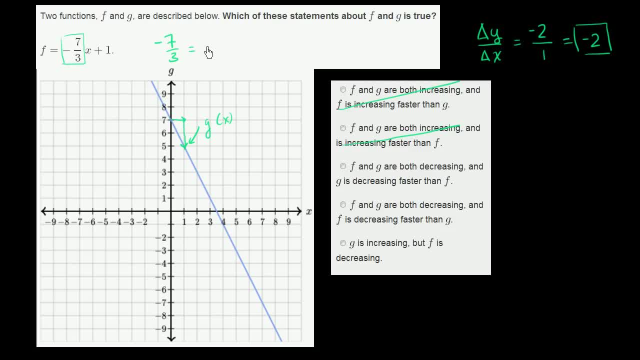 Negative 7 thirds is the same thing as negative 2 and 1 third. So f's slope Slope is more negative, So it is decreasing faster. So g is not decreasing faster than f. f is decreasing faster than g. So this is not right. 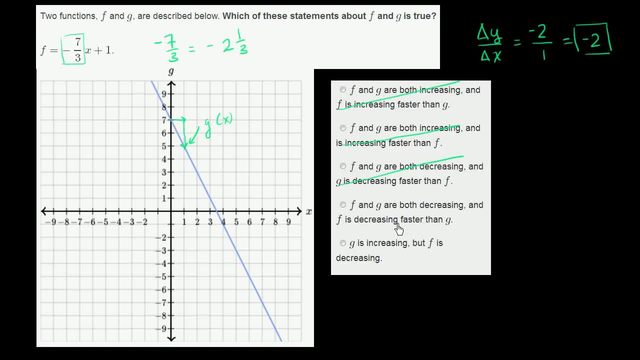 And then we have this choice: f and g are both decreasing And f is decreasing faster than g. This is right over here. We have this last choice: g is increasing but f is decreasing. We know that's not true. g is actually decreasing. 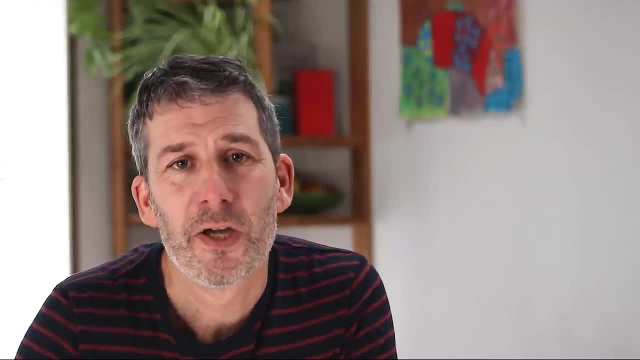 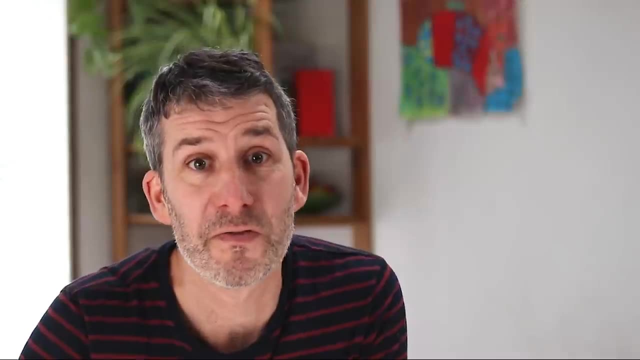 Hello, welcome to Maths Kitchen. Today we're looking at circle theorems. Questions on circle theorems come up regularly in the higher maths GCSE exams, so it makes sense to do a bit of revision on them in preparation for that. So today I'm going to go through each of the theorems and